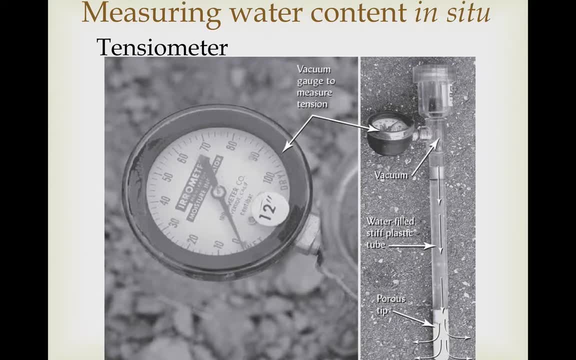 All right. so where I left off the last video, I was telling you about the tensiometer as a way of measuring water content. But one of the cool things about the tensiometer is it's not trying to measure water content as much as it is directly trying to measure metric potential. 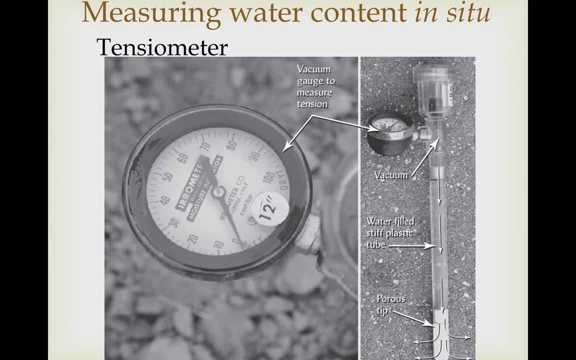 So that brings us back to the sometimes confusing world of potential, where we last were when we were talking about plant water potential. So before we dive into the details of how we figure out soil water potential and how we use it to tell us which way the water is moving, 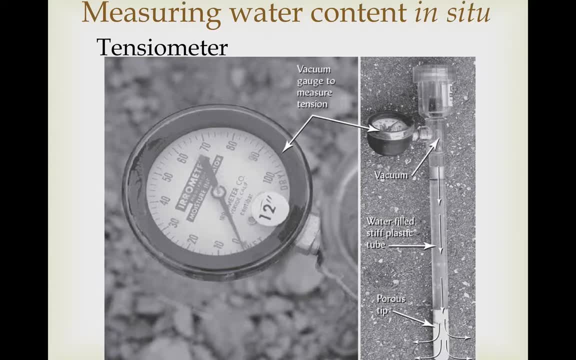 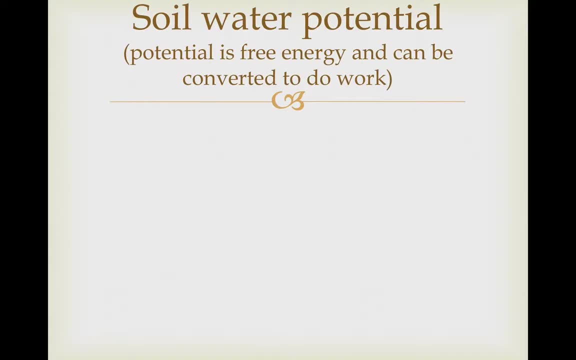 I wanted to step back for a minute and carefully define potential. So potential is free energy, and free energy is energy that can be converted to do work. So soil water potential, then, is telling us about the energy availability in the soil water that can do work of moving that water from one place to. 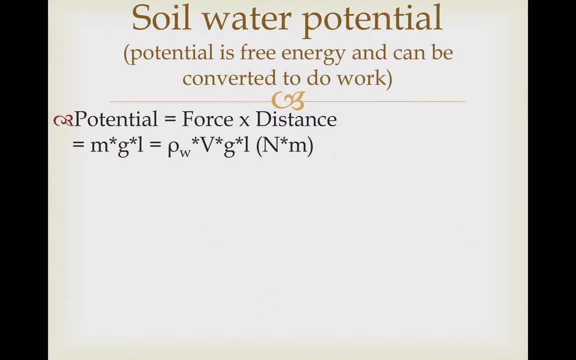 another. so work, then, is always force times distance. therefore, potential is force times distance. so force is a mass times an acceleration, and in this case our acceleration is going to be gravity and our distance is going to be a length. if we're talking about water, then we can take mass and we can make it the density. 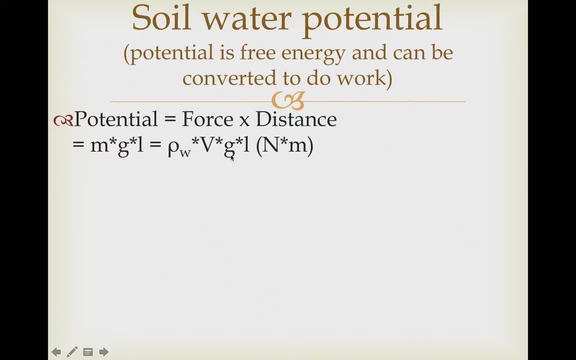 of water times, the volume of water, and then we still have our gravity and our length and this is going to give us units in the SI system of Newton meters. but sometimes we don't talk about potential. that way we normalize it or we divide it by something. so sometimes we talk about potential per unit weight of 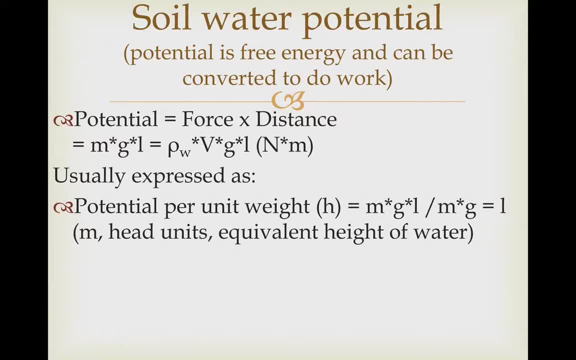 the water and that gives us units of meters, or this will be familiar to those of you who have taken hydrogeology, because this is units of head. so really, in hydrogeology, where you were talking about head, you were talking about potential. all right, so this is thinking. 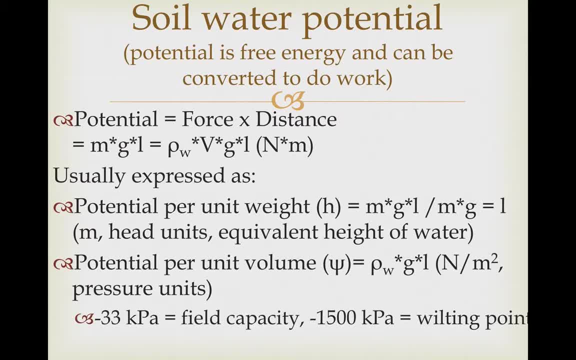 about the equivalent height of the water. we can also measure potential per unit volume. all right, and that will give us pressure units. so this is frequently used in the plant water potential and soil water worlds, because we can actually define some things in terms of potential. so remember, we talked about 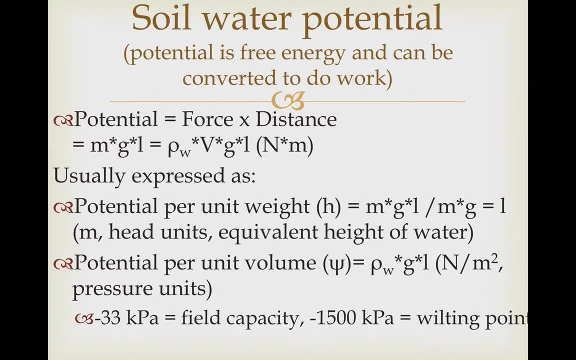 field capacity. so that is all the water that can be stored in a soil and not drain vertically due to gravity. well, that is often defined as occurring at negative 33 kilopascals. all right, and the wilting point- the point at which plants can no longer suck water out of the soil- is negative. 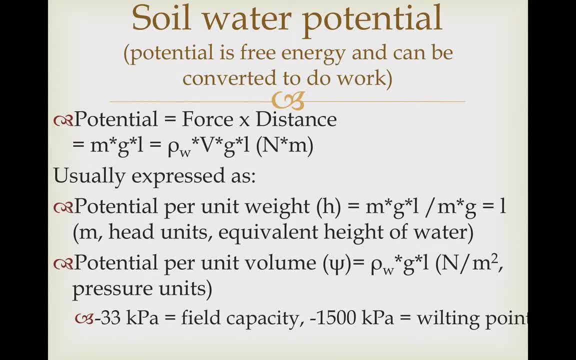 1500 kilopascals. in other words, the force with which plants can take up water is less than 1500 kilopascals. so if we get to a potential that is smaller than negative 1500 kilopascals, the plants can't counter that and they can't. 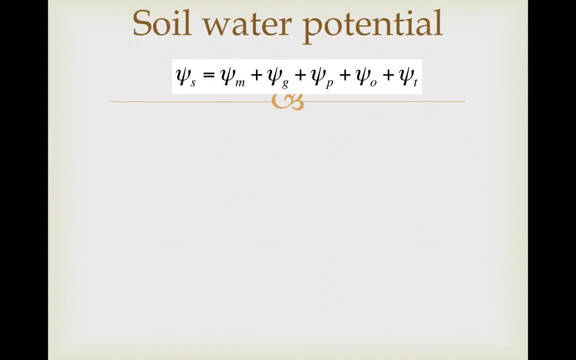 get it out of the soil, okay. so again, you saw an equation like this when we were talking about plant water potential, so potential psi. so we have psi s is the total soil water potential. and now we're going to break down each of these terms, which actually you have seen before, when 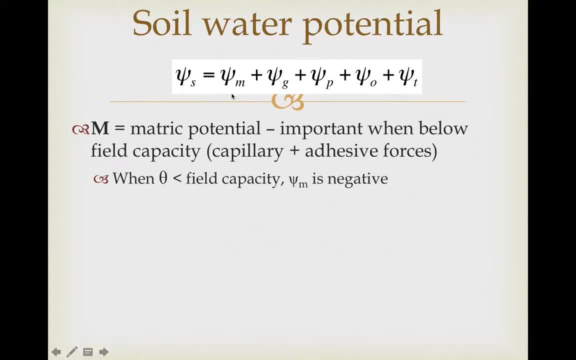 we did this for plants. so psi sub M is the matrix potential. again, this is our tension or our suction forces. so the matrix potential is important when the soils are below field capacity, so when all of the water is being held in place by capillary and adhesive. 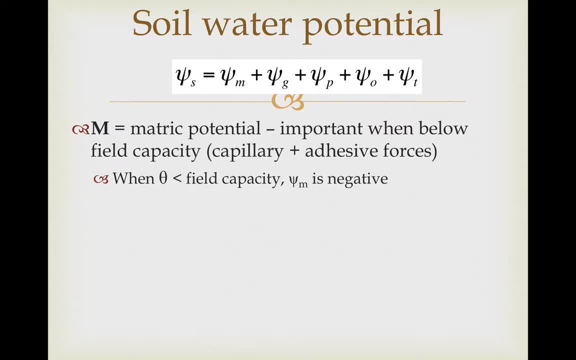 forces. so when the water content is less than field capacity, the matrix potential is going to be negative. when the water content is at or above field capacity, the matrix potential, or the tension that's holding that water in place, is going to be zero- the gravitational potential. so again for our hydrogel. 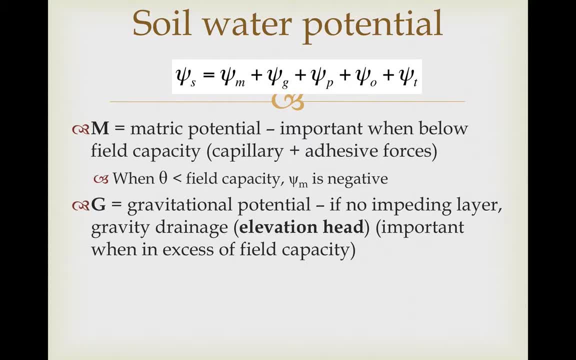 in the group. this will be familiar because it's elevation head. so this is what sort of gravity drainage we will get if gravity is just free to act on any of the water that's not held in place by capillary and adhesive forces. so this is important when we have water contents that are someplace between 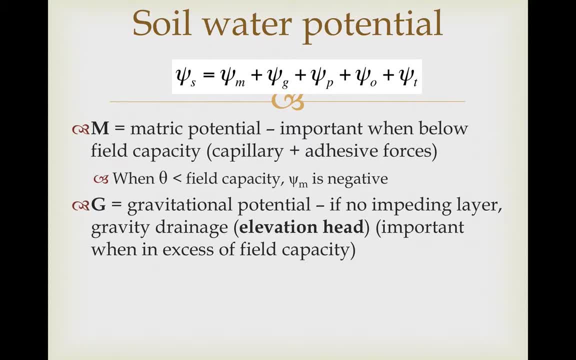 field capacity and saturation. the third main potential we're going to think about in soils is the pressure potential, and this is really only important in saturated conditions and this hydrogeologist is equivalent to our pressure head. so if we have to review, if we are in less than field capacity, 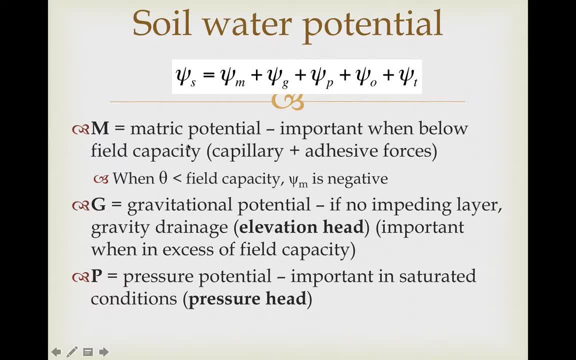 conditions, we're going to mostly be concerned about matric potential. if we're between field capacity and saturation, we're going to be mostly concerned about gravitational potential. and if we are, you know, if we're in a situation where we're in a situation where we're in a 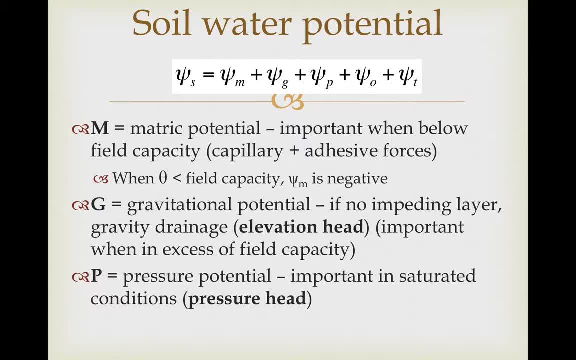 are at saturated conditions. now we're in the realm of hydrogeology and we're going to care about pressure, potential and gravitational potential. so if we measure all three of these things, we can tell ourselves, we can get information about what range of conditions the soil is in and go from there. there are two. 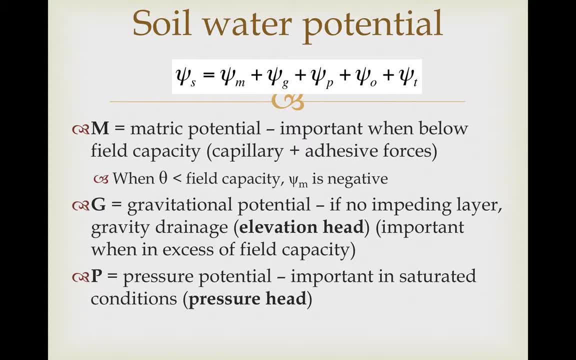 other terms in that equation and in most cases these are going to be small potatoes compared to the rest. but Psi O is the osmotic or solute potential. now you can imagine some places where this is important. this might be important if you have some salinization happening in your soil, moisture or groundwater, and T is thermal. 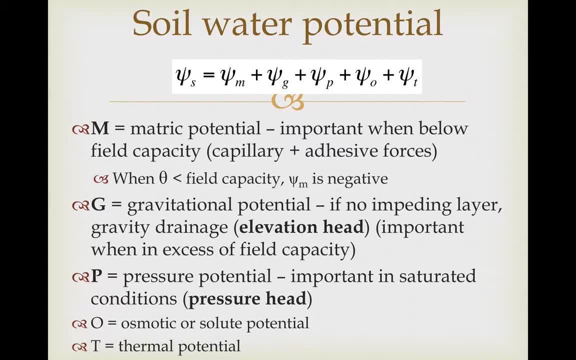 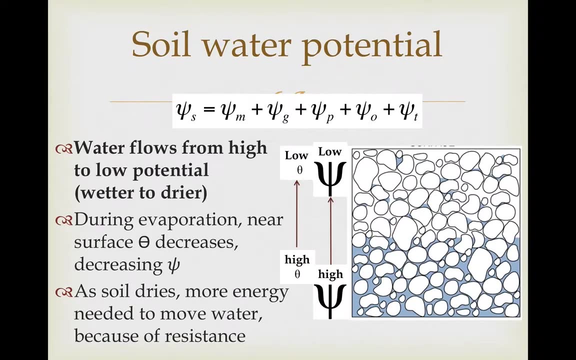 potential. so, just as touching back to plants, osmotic or solute potential was really important in plants, and thermal potential is that one that we keep sort of writing into the equation and then crossing off in almost every case. okay, so we've got our equation and you should remember from talking about plants or 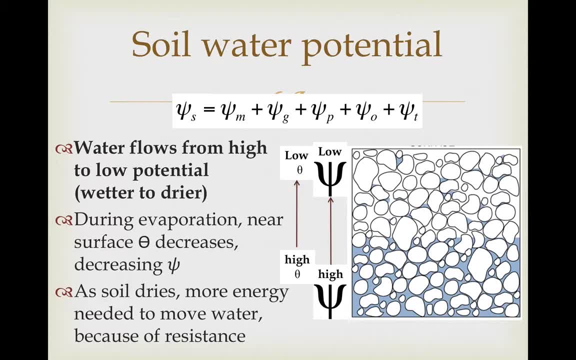 from taking hydrogeology, that water is going to flow from areas of high potential to areas of low potential and in in soils. this is going to be from areas that have a high water content to areas that have a low water content. now, when I say it flows, that doesn't necessarily mean it does it. 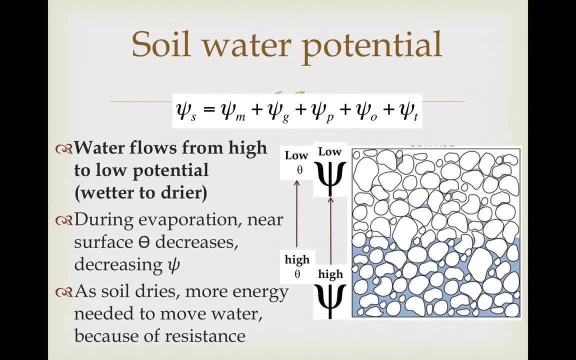 completely of its own volition, just under the influence of gravity, because, remember, gravity is only going to be at play if we are in excess of field capacity. but in this case we have wet soils down here and we have dryer soils up here, so we have high potential and high 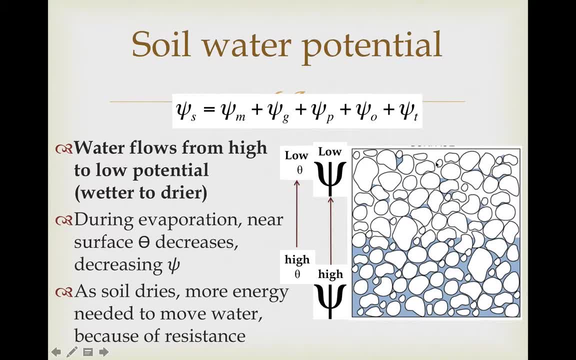 water content down here and low potential and low water here. so water should be moving from this wet area up to and through this drier area. so this is what the situation we find ourselves in when we are evaporating water. so our near surface water content has been decreased by. 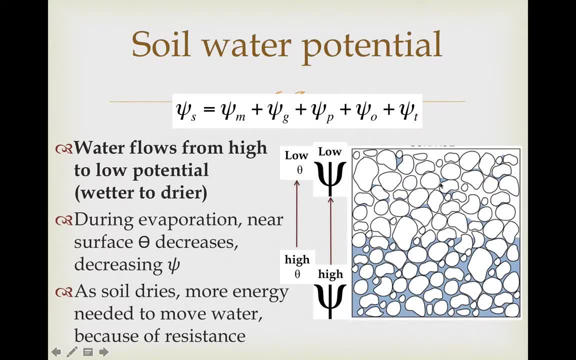 evaporation so that decreases the water potential up here. down here there's still plenty of water available. so we've set up a potential gradient and water that is being evaporated from here and out is going to tend to be pulled from this high potential area down at the base of the soils into the lower. 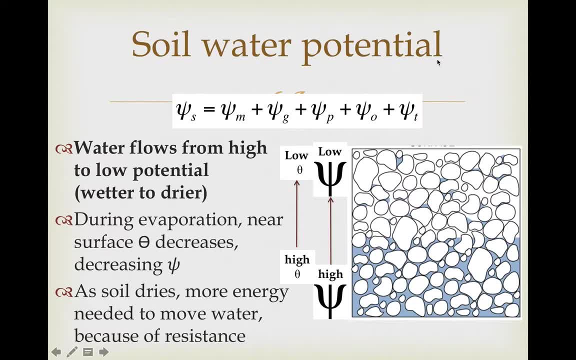 potential area and then ultimately into the atmosphere. of course, if you remember, from evaporation as the soil dries out, more energy is necessary to make it easier for the soil to slide down to the bottom of the pot and be able to move that water. um, because there's a lot more resistance in the in the equation. uh, when we're 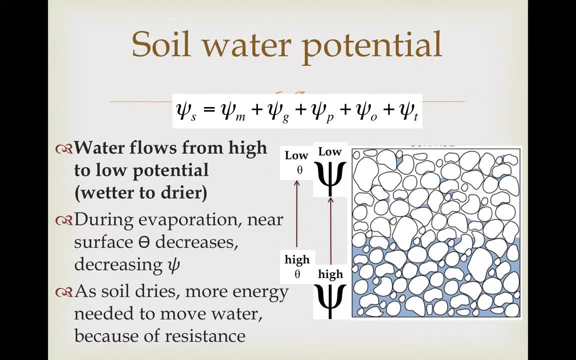 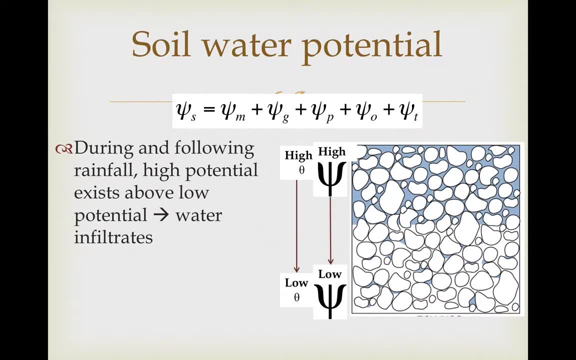 trying to move through air-filled pores in that evaporation process and and a longer distance of air-filled pores. all right, we could flip our diagram on its head. so, during and following rainfall, water is being added to the surface of the soil right, and so we get a high water content. 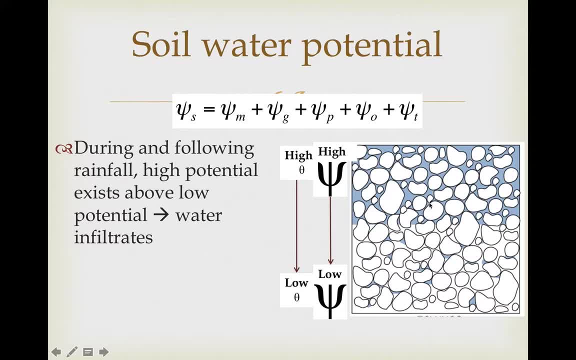 and a high potential up here, and that is going to bring water, uh, down to the lower parts of the soil because they have a low water content and a low potential. so, again, gravity is going to be part of this. in this case, it looks like the surface of the soil is saturated, so we 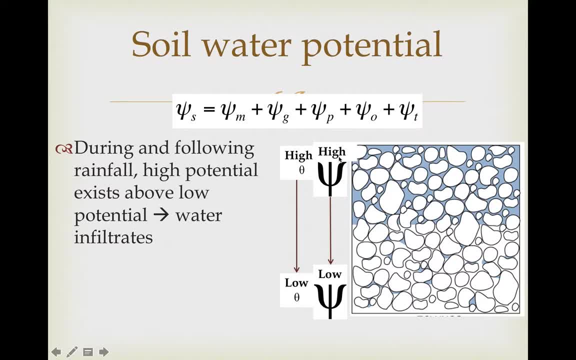 have a high water content and a low potential, so we're going to be adding water to the lower to think about some gravitational head and maybe some pressure head. but down here we have only matrix potential to think about, because I'm just gonna guess that this is under field capacity and, remember, matrix potential is going to be. 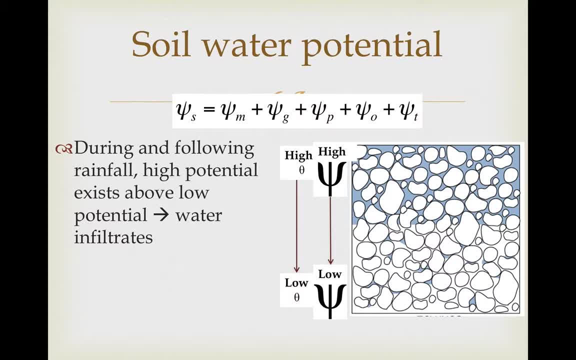 negative because it's a suction, and so we have positive gravitational potential and pressure potential up here and negative potential down here. so water is going to move from the high potential area to the low potential area and that, right there, is the basis for infiltration. but before we dive into, 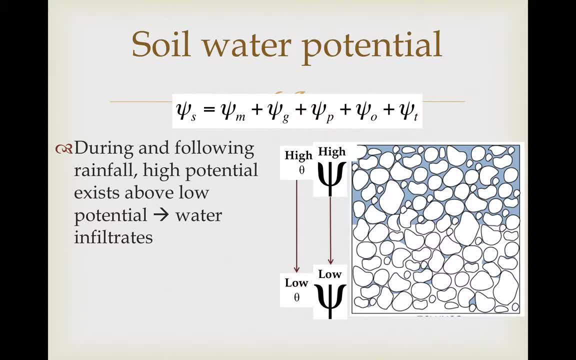 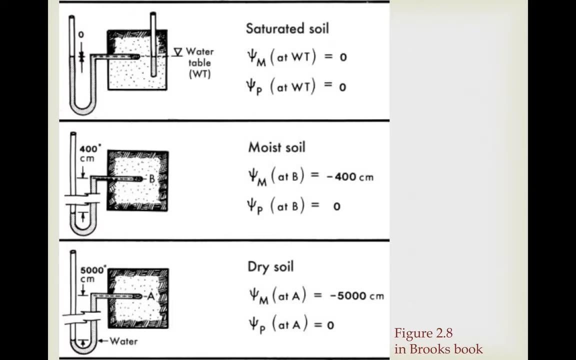 exactly how infiltration works, which is what we'll talk about on Thursday when I'm back in class. let's spend some more time thinking about what we can tell from these potential measurements about what's happening in the soil. so this is a diagram from your book. what we've got going on over here is a. 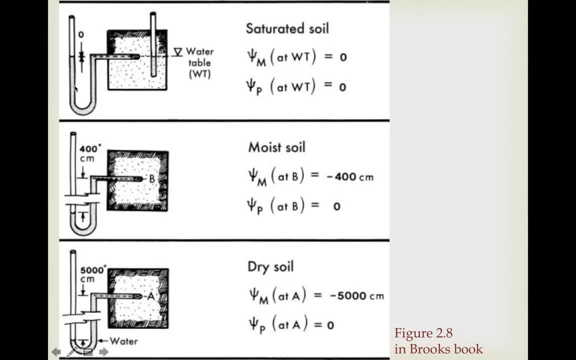 measurement of the surface of the soil. and the surface of the soil is a manometer, so that's measuring the pressure and it's supposed to be measuring the pressure right here in the soil. and I said pressure, remember we're talking about potential in pressure units. so if we have and and this right. 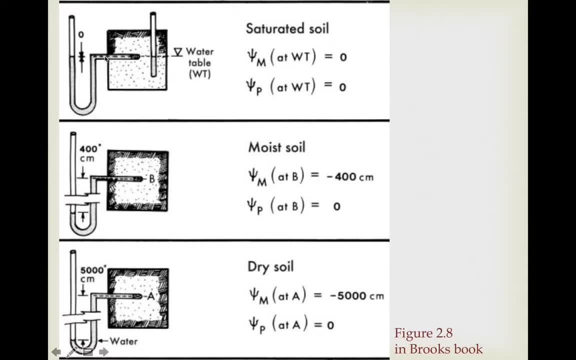 here is a well and that well is saying that the water table is right here in this block of soil where the manometer happens to be measuring. so we are sitting right at the water table, so our matric potential at the water table is zero and our pressure potential at the water table is zero. 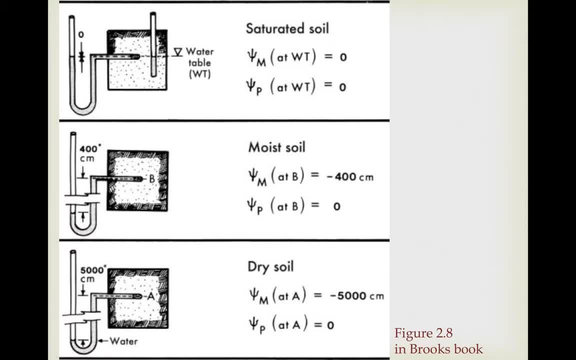 because there's no weight of the overlying water. so the only potential we would have to think about here is the elevation potential. so opportunity, and that is just going to be dependent on the elevation that our manometer is at. if we take a moist soil- so notice, it says moist and not saturated. if we take 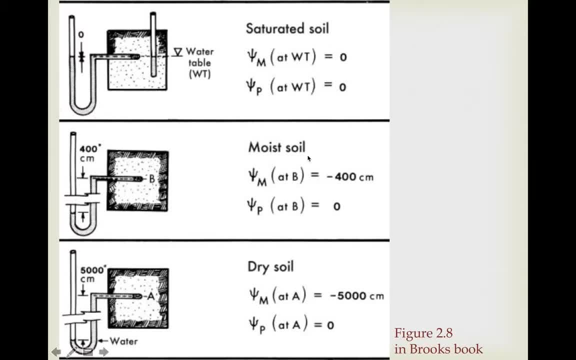 a fairly wet soil. now we have a matrix potential and again it's negative, and notice the units here of centimeters. that means we're gonna be expressing it in terms of head, so it's still a potential, but we're just using head units here. so it's negative 400 centimeters because there's no weight of. 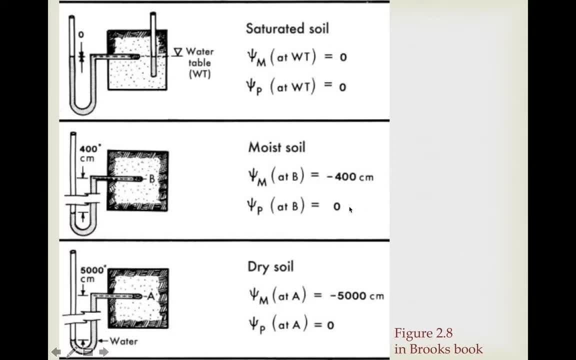 overlying saturated water, our pressure potential is going to be zero and again our gravitational potential is just going to reflect the elevation. if we dry that soil out, our pressure potential stays negative. but now our matrix potential, or the suction, gets really small, negative, 5,000 centimeters all. 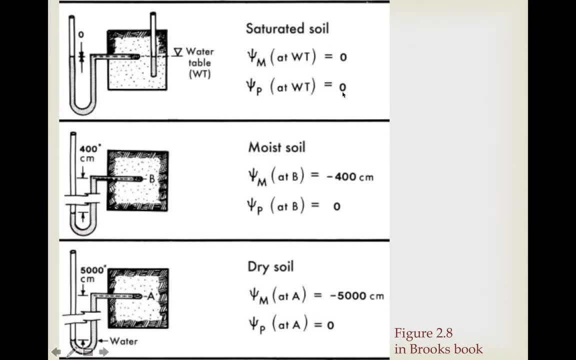 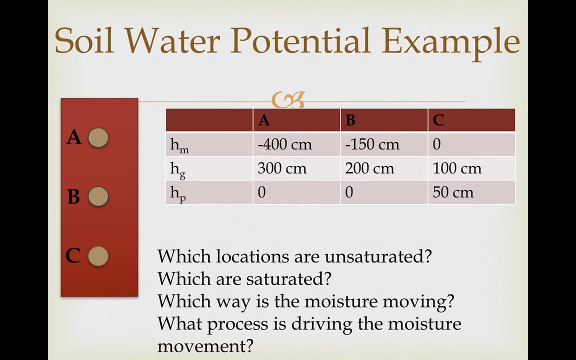 right. so in this scenario, our saturated soil has the highest potential, at zero. our moist soil has a slightly lower potential- negative 400 centimeters- and our dry soil has the lowest potential, at negative 5,000 centimeters. all right, so here's my version of that. so we've got a soil profile and we've 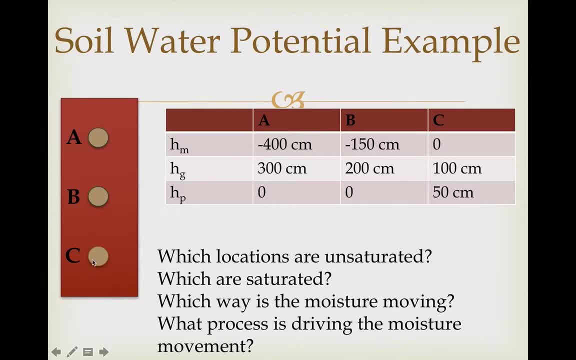 got potential measurements of three different depths in the soil profile. all right, a, B and C. And here's the data. So this is- and again I'm going to use head units. so this is the metric head, the gravitational head and the pressure head. So at A we have a metric head of. 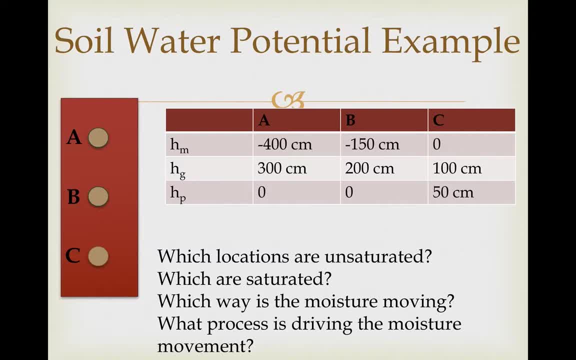 negative 400 centimeters, a gravitational head of 300 centimeters and a pressure head of zero. So if we're over here at B we see a little bit of a less negative metric head. It's at a lower elevation, so that head has gone down as well and it's still at zero. If we get down to the 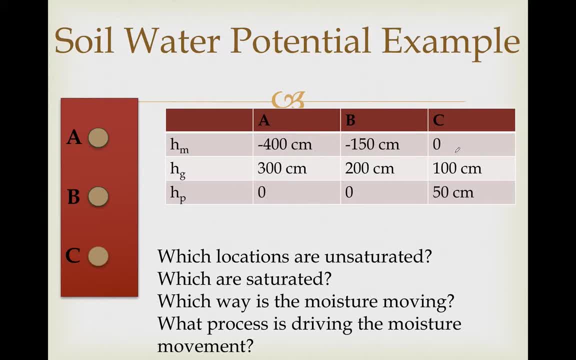 bottom of this soil profile, our metric head is zero, our elevation head has gotten a little lower and our pressure head has gotten a little higher. So the first question I want you to think about here is: based on this data, which locations are unsaturated? 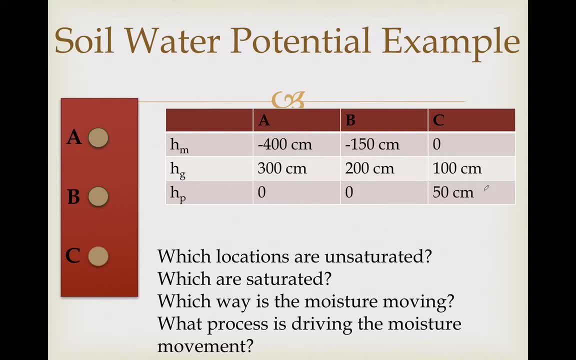 The key thing to look at if we're thinking about identifying saturated versus unsaturated conditions is whether we have a pressure head And at C we have a positive pressure head. So we know that C is saturated. At A and B we have no pressure head. 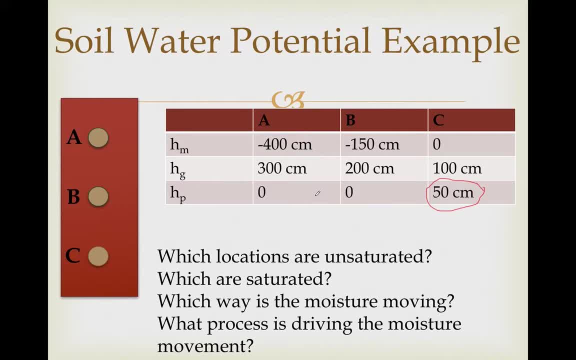 so now we're unsaturated or we're sitting right at the water table. But we know we're not sitting right at the water table because we have these negative metric heads here at A and B. All right, And if we were sitting right at the water table they'd be zero. 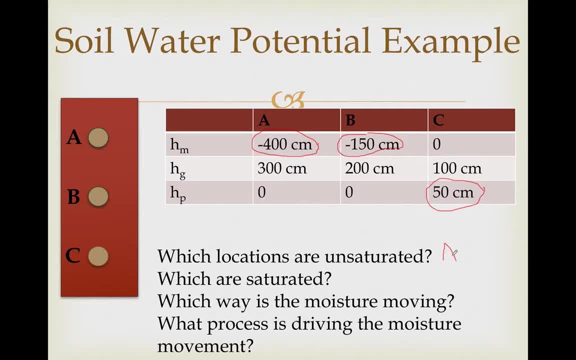 So my answer to this first question is that A and B are unsaturated. Which locations are unsaturated? Let's look at the second question. So which locations are unsaturated? Which locations are unsaturated is saturated? Oh, I already answered that It's the one with the positive pressure head. 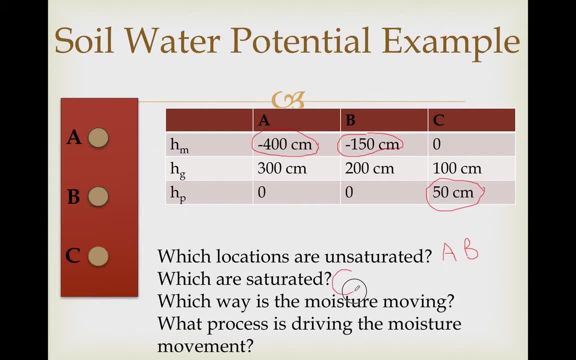 and a zero metric head. All right. So the next question is: which way is the moisture moving? In order to answer that, we need to know about the total head or total potential in each of these locations, And we can do that by adding up the numbers of the different head components. 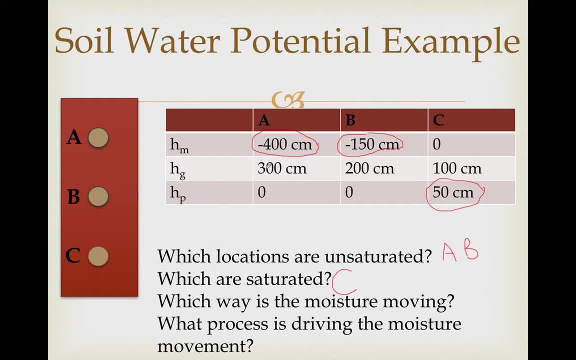 All right, So at A we have negative 400 plus 300 is negative 100 centimeters. At B we have negative 150 plus 200. That's a positive 50 centimeters. And at C we have 100 plus 50. So our total head is 150 centimeters. 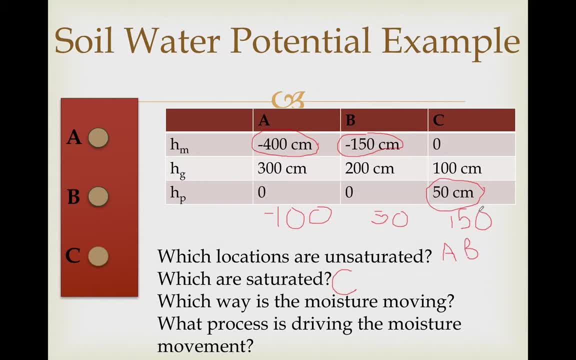 All right. So our water is always going to flow from high head to low head, which means it's going to flow from C to A, And C to A means it's going up, right. So which way is the moisture moving? It's moving up, All right. That's fairly simple math, hopefully. 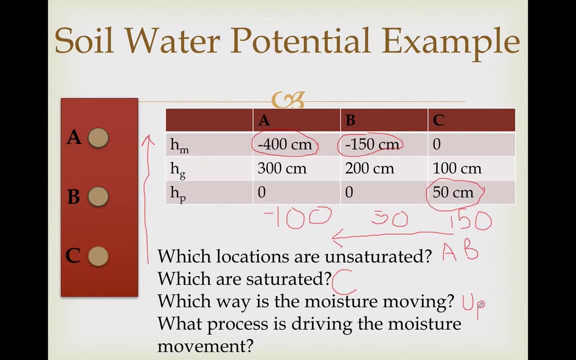 So now let's bring it back to hydrology. What process is driving the moisture movement? What brings water vertically up in a soil profile? You should be thinking to yourself: evaporation or evapotranspiration, All right. So that's an example of how we can use soil water potential data to answer some pretty basic. 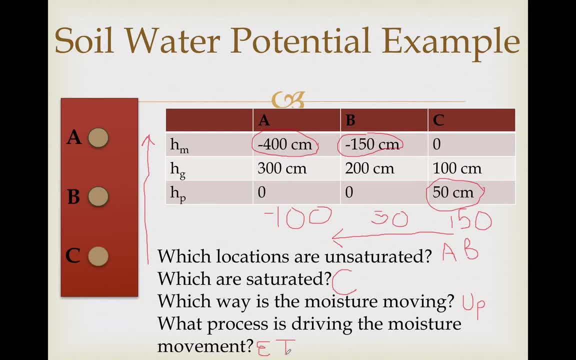 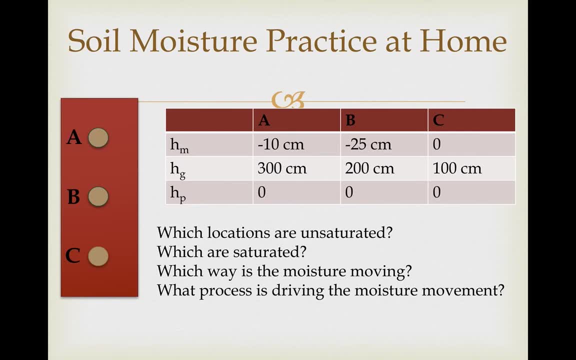 questions about what's going on hydrologically within a soil profile. So what I want to leave you with today is a different set of data, same cartoon, but the numbers in the table have changed, and I want you to be able to answer the questions about which locations are unsaturated, which are? 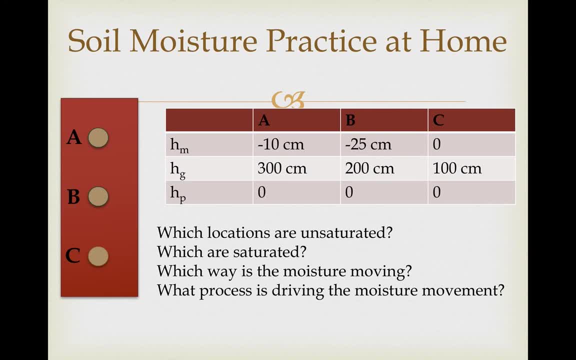 saturated, which way the moisture is going and what's driving the moisture movement. So work this answer out on a sheet of paper and then head to the practice set home folder within Blackboard and you will be able to check your work And I will see you on. 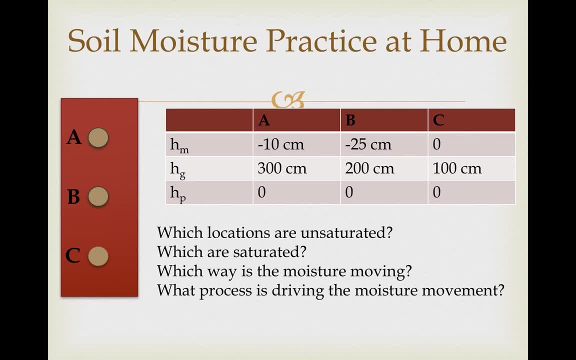 Thursday, where we'll take these ideas of potential gradients and soil moisture and we will integrate them to understand the process of infiltration. 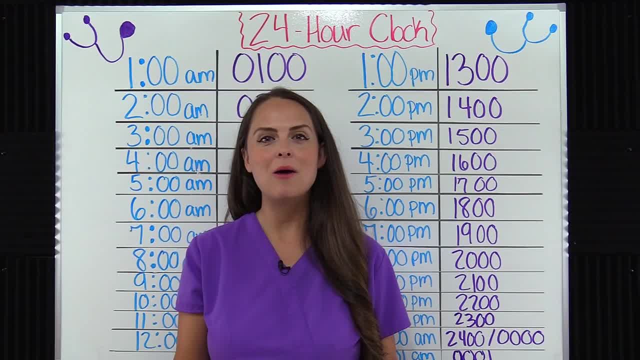 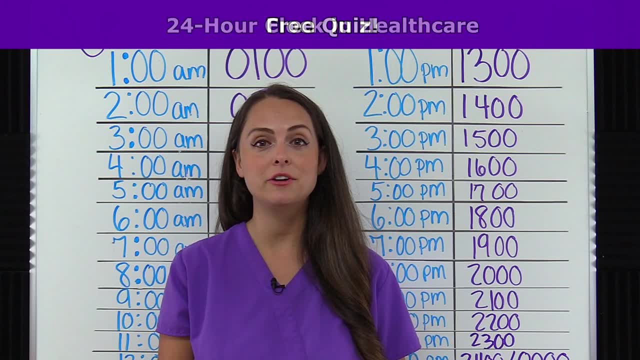 Hey everyone, it's Sarah with RegisteredNurseArienecom, and in this video I want to be talking about the 24-hour clock that we use in health care. And whenever you get done watching this YouTube video, don't forget to access the free quiz that will test you on this content. 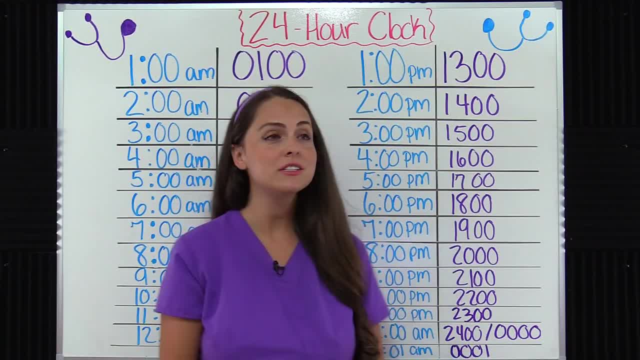 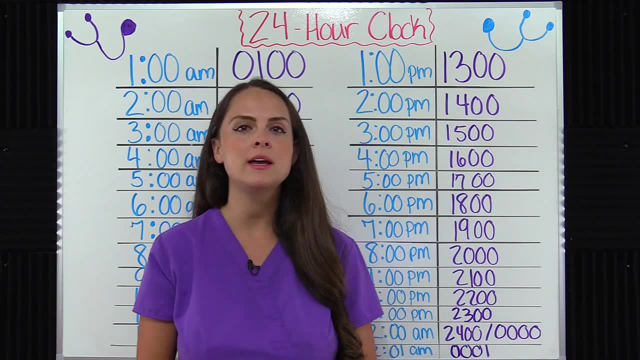 So let's get started. In most health care facilities, nurses are required to follow the 24-hour clock, which most people know this as military time, rather than following the 12-hour clock, which is am and pm times. 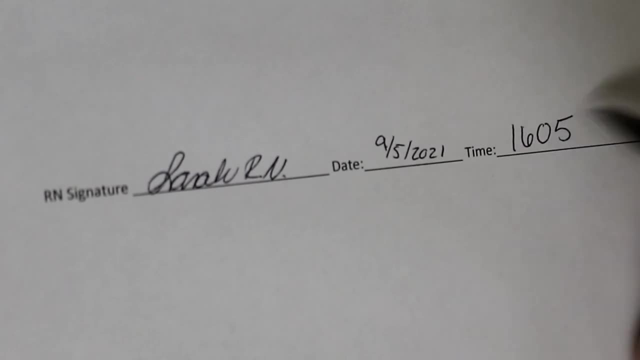 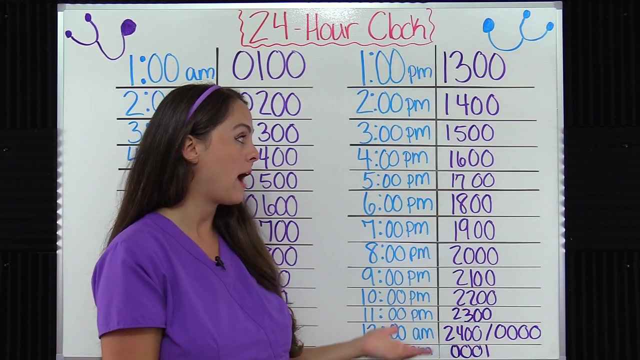 Now, as a nurse, you are going to be dating and timing things constantly And whenever you're looking at the medication administration record, it's going to be giving you times in the 24-hour format for whenever you need to administer medications. So it's really important you're familiar with this. 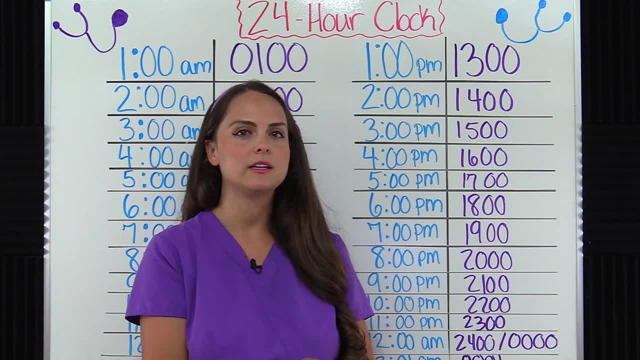 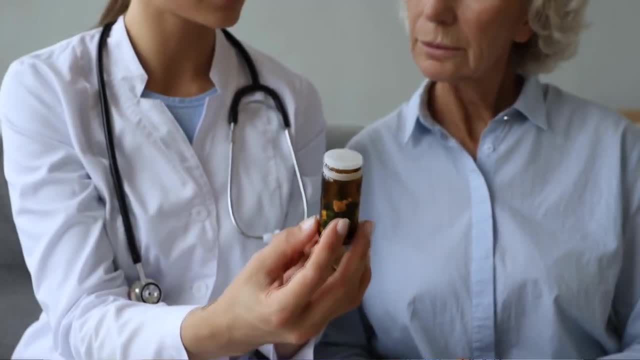 Now, why do we use the 24-hour clock in most facilities than the 12-hour clock? Well, we want to prevent errors. So, for instance, let's say a patient needs a medication at 4 o'clock. Well, it's not good to write the medication at 4 o'clock. 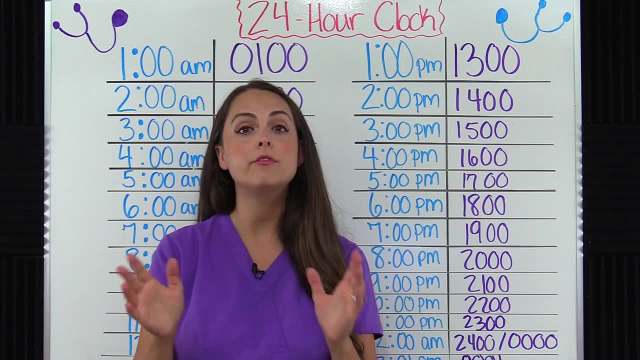 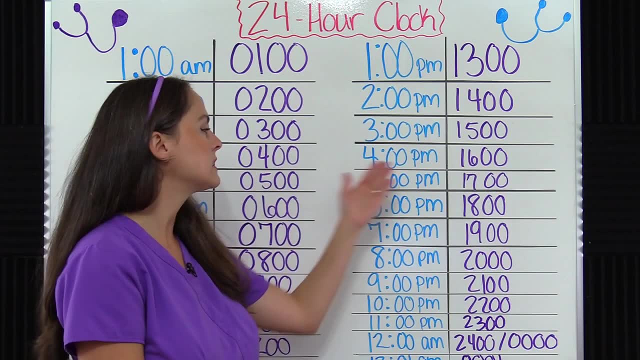 The medication needs to be given at 4 am or 4 pm, because that could cause room for error. Instead, the provider or the pharmacist can put in 0-400 hours or 1,600 hours, And those two numbers are completely different, so that helps prevent errors. 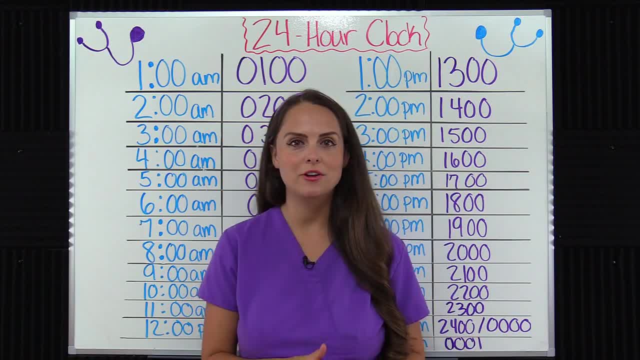 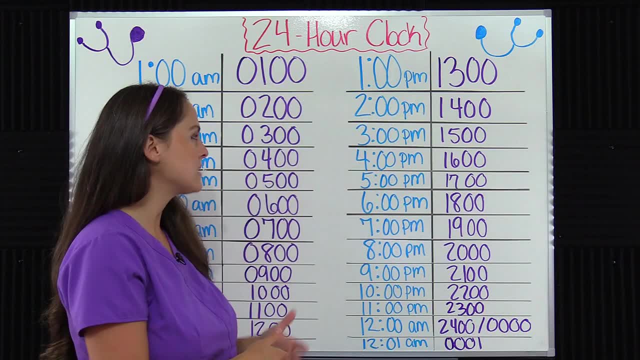 So now let's look at the 24-hour clock versus the 12-hour clock. Here on the board I have the first 12 hours of the day, which are the am hours, And then over here I have the last 12 hours of the day, which are the pm hours. So first let's look at those first 12 hours of the day. Whenever you convert it over to the 24-hour clock, it's very, very simple. You just look at the time and either put a zero in front of the number or just rewrite it without the colon. 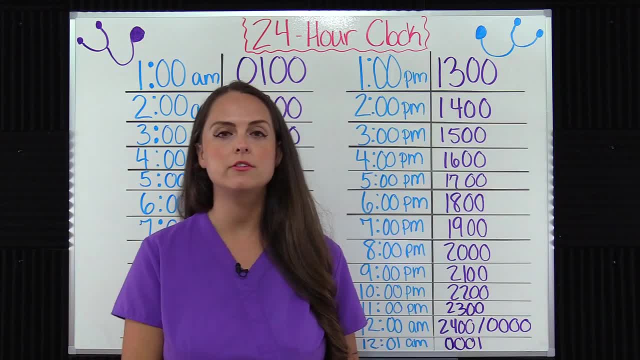 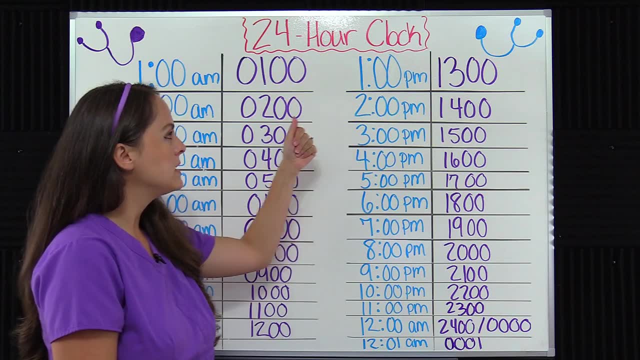 And it's 1,200 hours. Then we flip over to the last 12 hours of the day And this is where it takes a little bit of work on your part. So 1 pm is going to go to 1,300. 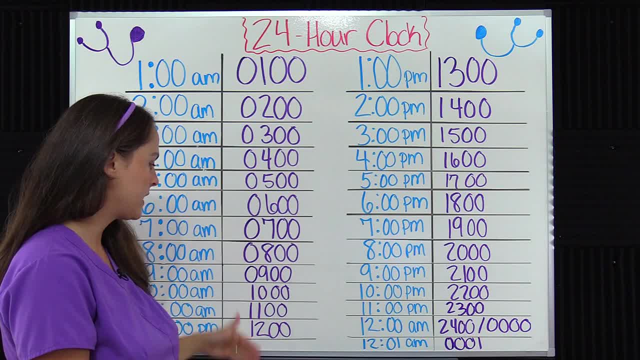 Because, remember, we're going to 24 hours, so it's just going to keep on counting. So, over here we're over at 12.. Now we're over at 13. And then 2 pm is going to be 1,400 hours.